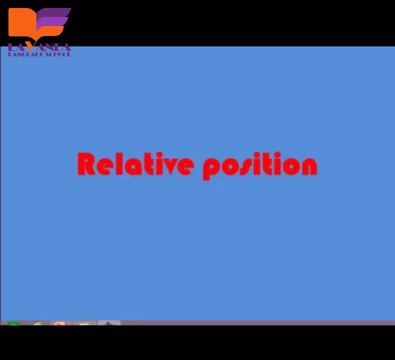 How are you, my lovely, dear students? I hope you are fine. Today we are going to know about relative possessions. Relative possessions means the relationship between two words And in this lesson we are going to learn each word and its opposite. Let's start. 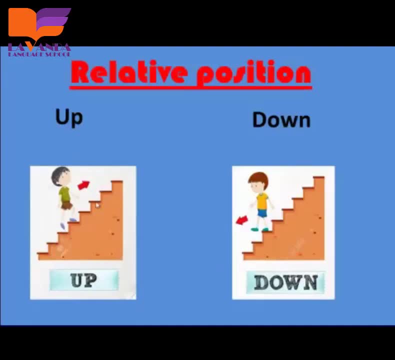 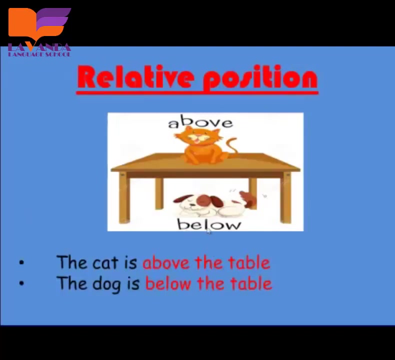 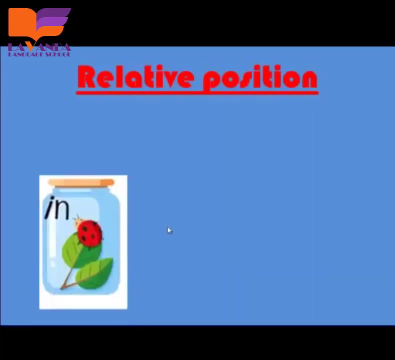 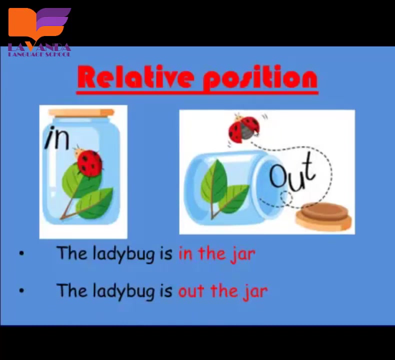 In the first picture, the boy is going up the stairs. The second one, the boy is going down the stairs. Let's see another two words. The cat is above the table, But the dog is below the table. Okay, The ladybug is in the drawer. In the drawer. Oh, oh, Now the ladybug is out the drawer, Out the drawer. 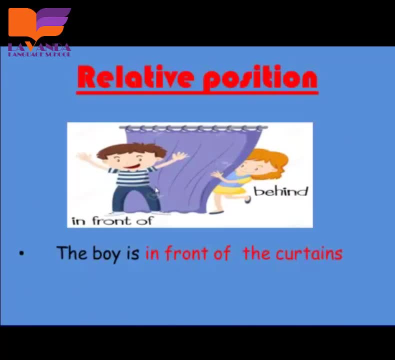 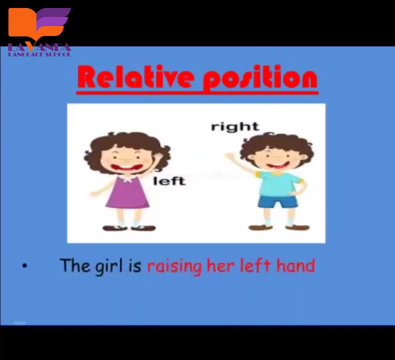 The boy is in front of the curtains, In front of the curtains, But the girl is in the front of the curtains, In front of the curtains, But the boy is behind the curtains. Behind the curtains, This girl is raising her left hand, Left hand, But the boy is raising his right hand, Right hand. 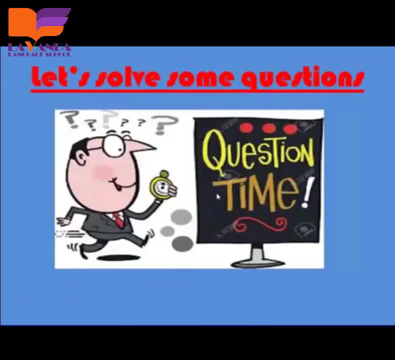 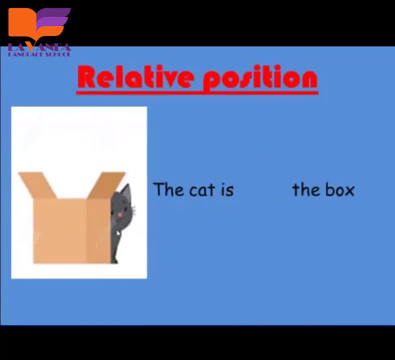 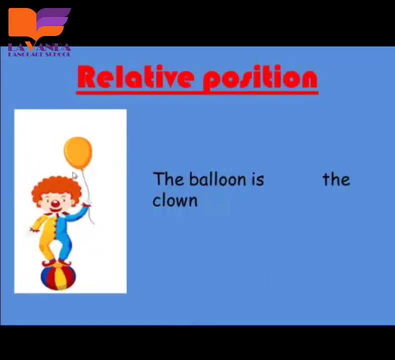 I hope you are understanding the words. Let's solve some questions. Where is the cat? The cat is what to the box? Yes, Super Is behind the box. Okay, So the box is in front of the cat. Super The balloon is what to the clown? The balloon is, Yes, Above the clown. 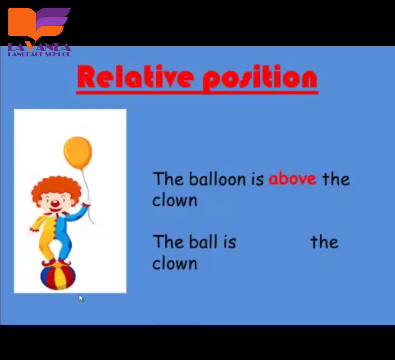 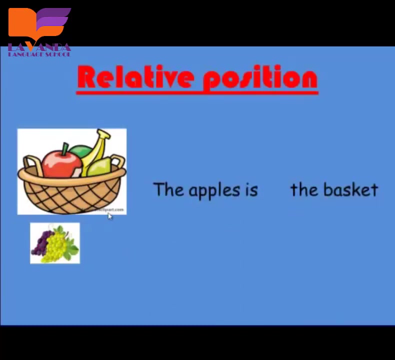 Wow. But the ball is what to the clown? The ball is Below the clown. Super Yummy Fruits. Let's see Where is the apple. The apple is what to the basket? The apple is in the basket. Super.